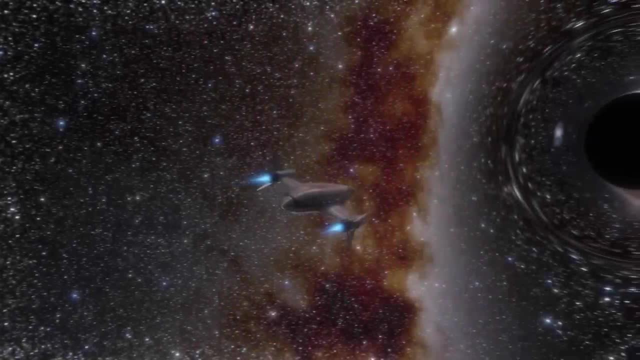 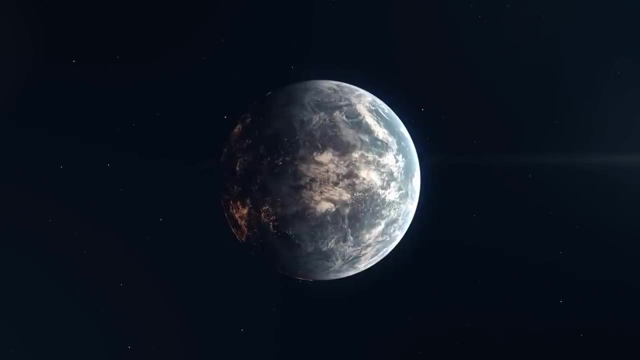 extraordinary planets. But before we get into the details, let's take a look at the star system. Before we start, we would like to invite you to actively participate in our channel. We welcome comments that provide a valuable contribution to the topic and are also 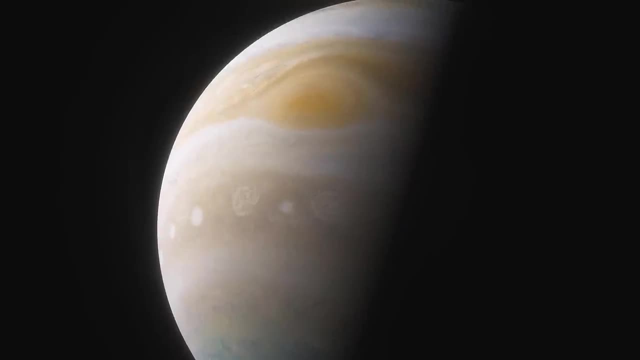 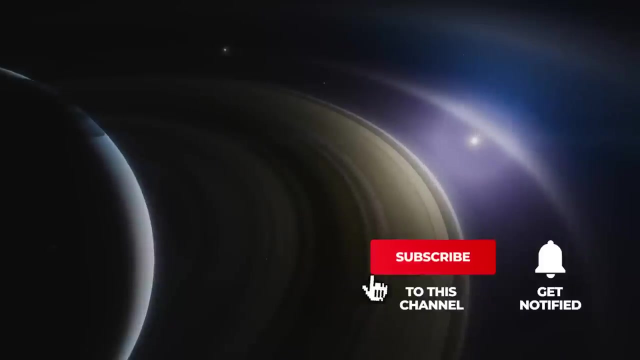 interesting for others. In the future, we will reward our subscribers with a heart and a comment pinned to the top. Make sure you've subscribed, write it down at the beginning of your comment and the best and most beautiful comments will get a special award from us. 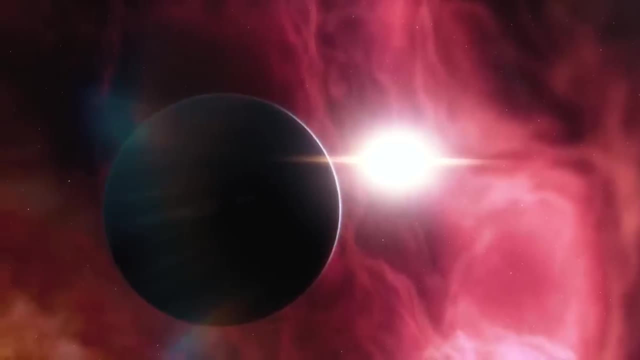 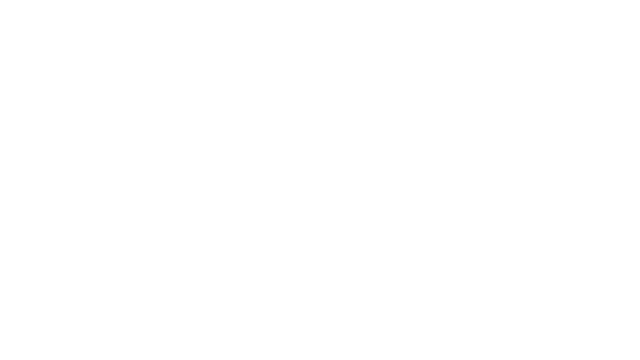 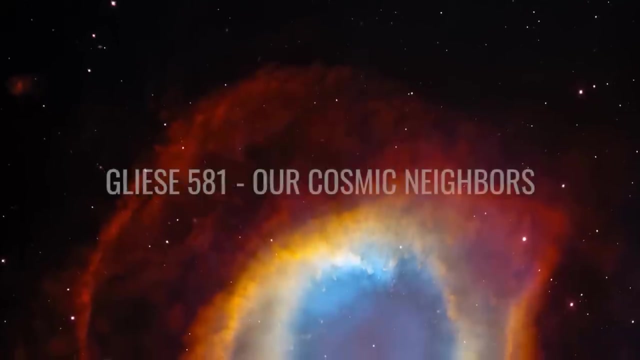 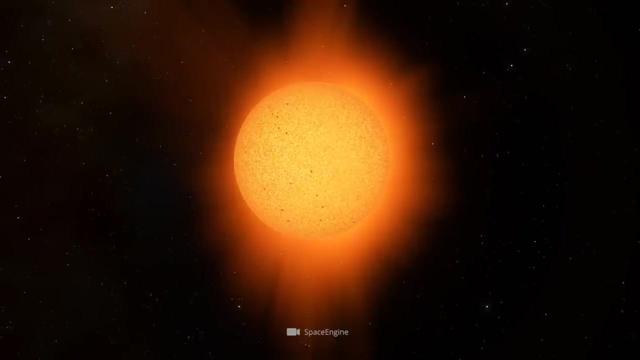 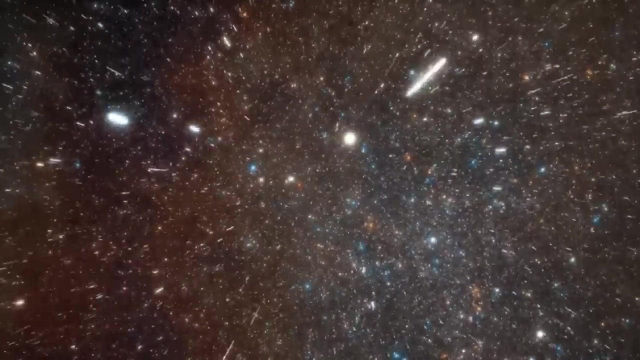 We are now going on a journey to the Gliese system together: Gliese 581, Our Cosmic Neighbors. The star Gliese 581 is not one of our closest neighbors, but with a distance of about 20 light-years it is still around the corner on a cosmic scale. A spacecraft would have to travel. 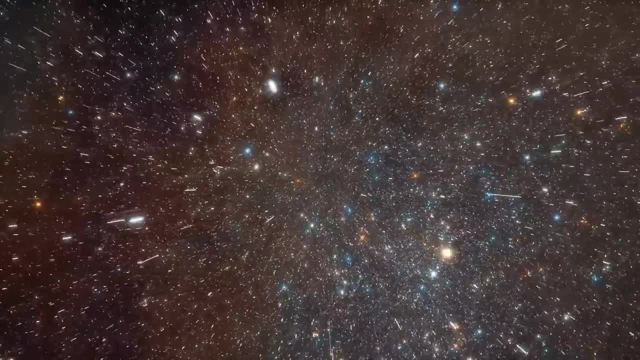 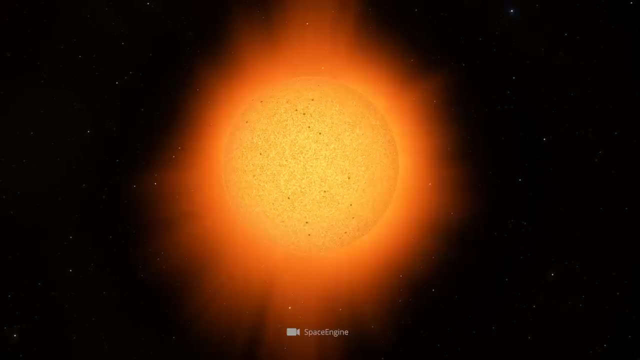 100 miles per hour to reach it. The star Gliese 581 is not one of our closest neighbors but with a 190 trillion kilometers and head towards the constellation Libra to reach the comparatively faint red dwarf and its planetary system, A star of spectral class M3V, Gliese 581 is about 100. 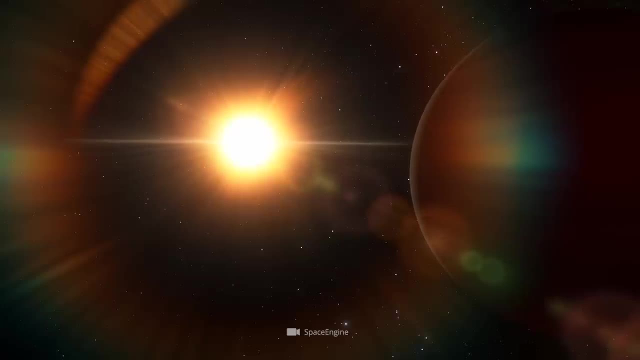 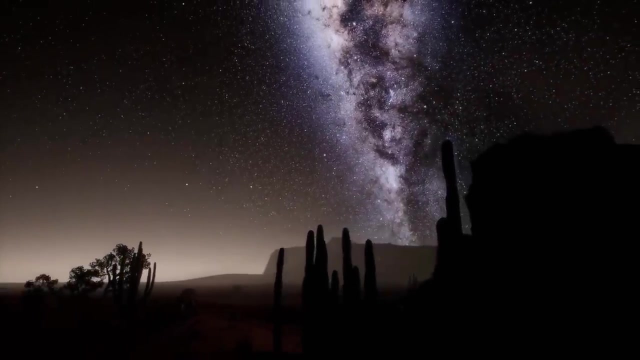 times fainter than our Sun and has only about 21% of the mass. In 2005,, researchers first announced that they had detected an Earth-like planet in the Gliese system. According to initial observations, the exoplanet was about two or three times. 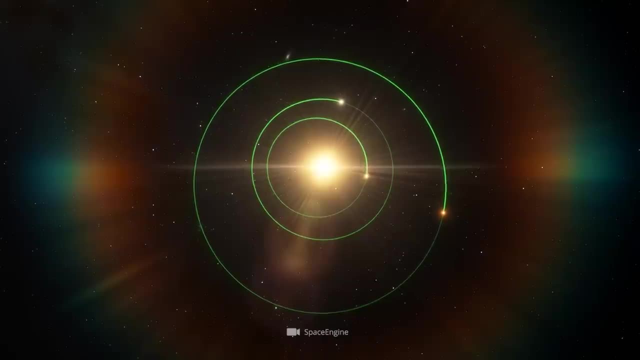 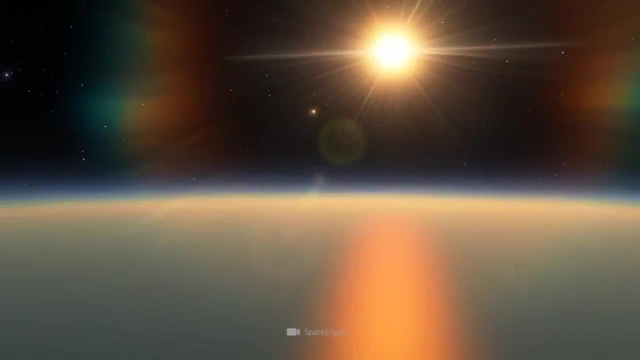 the size of our Earth. Scientists calculated a slightly higher gravity than ours and determined that this planet was in the habitable zone of its star, so it should be close enough and far enough away to get enough light and heat, but still have a temperate climate. In the world of. 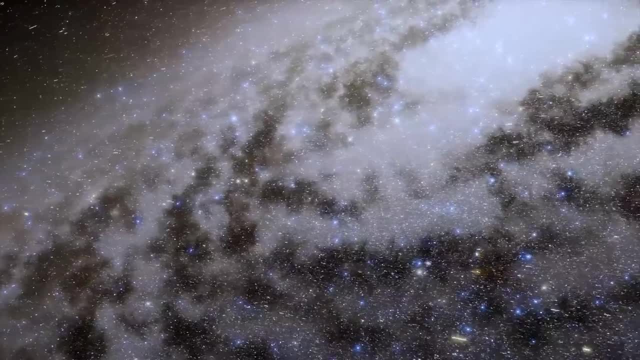 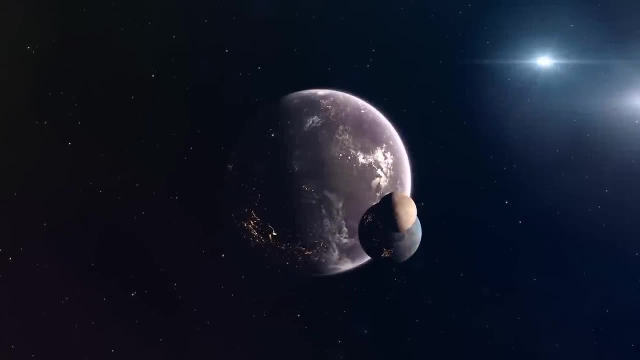 astronomers and cosmologists. this news caused excitement. The search for exoplanets is a field of science that is still quite new. Only since 1995 do we have the ability to detect planets outside our system. The impact of the exoplanet on our planet is enormous. The exoplanet is a 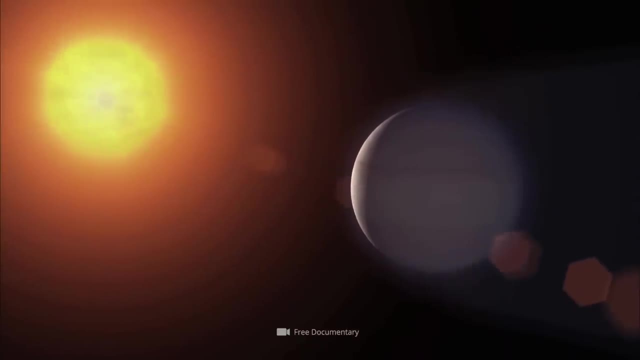 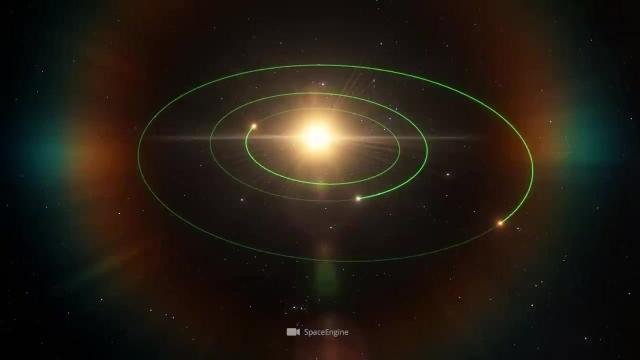 planet that has proved possibilities to find the tiny and dark planets in space suddenly increased the probability to find traces of extraterrestrial life in the foreseeable future. After the announcement of the success, the Gliese system was studied meticulously for years and some strange 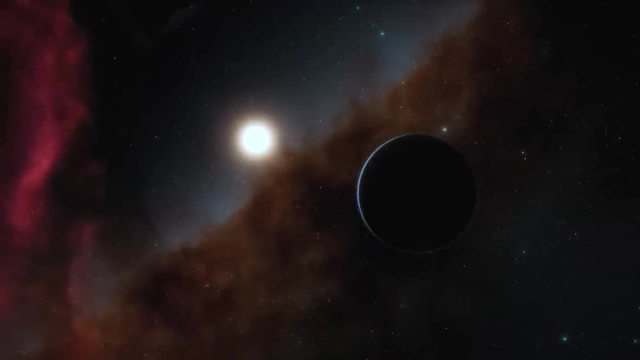 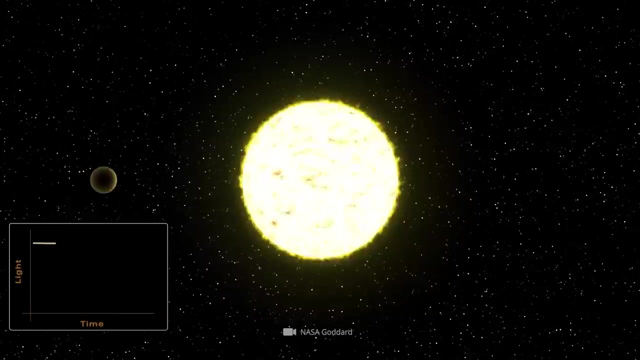 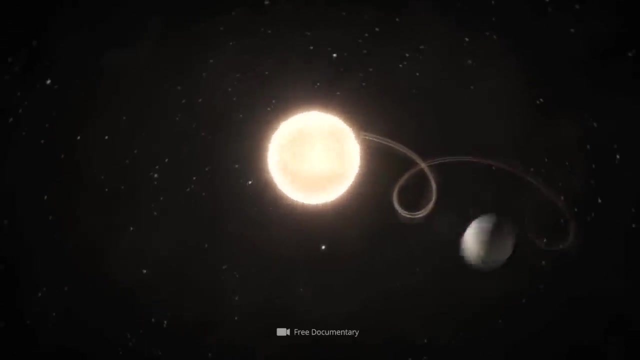 things happened. Only a few months after the discovery of the first exoplanet, four to five more planets were spotted. The exoplanets were not discovered by means of the transit method, with which planets pass as tiny dots in front of their stars, but by a statistical method which detects exoplanets by slight shifts in the proper motion. 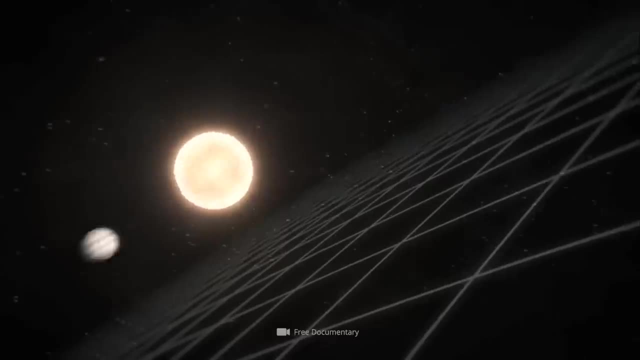 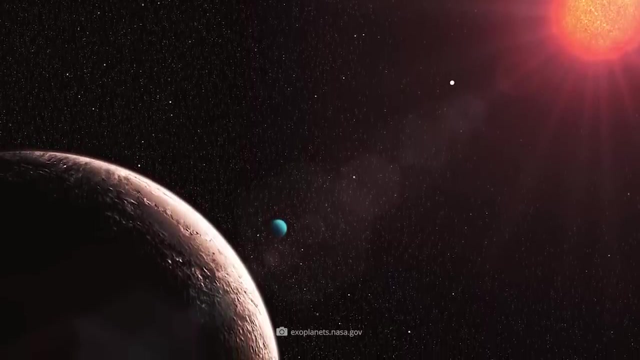 of the star Planets provide by their gravity for the fact that even large and massive stars come a little into the spin. All planets discovered in the Gliese system were determined in this way, and exactly here lies apparently the problem, because research groups from the whole world 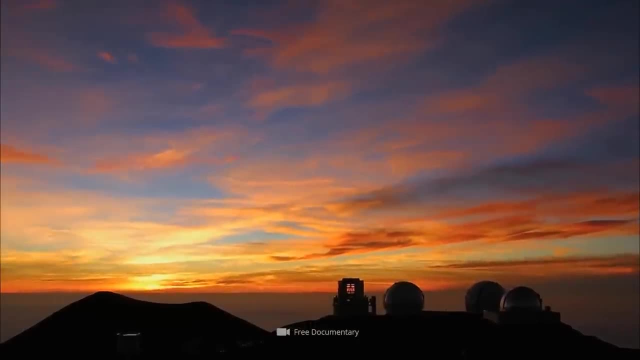 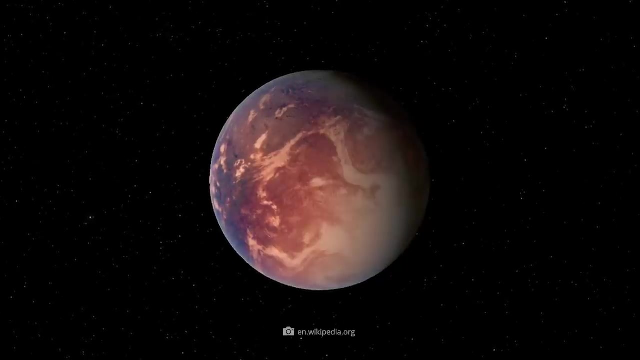 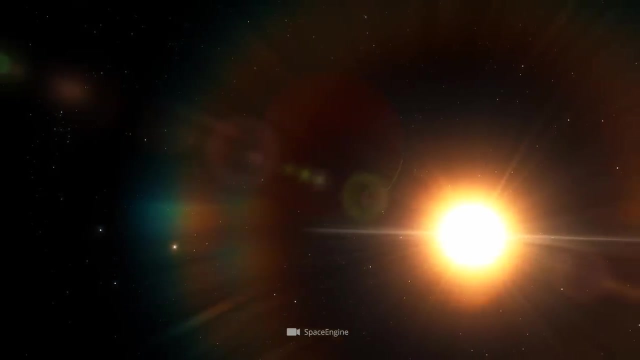 came partly to fundamentally different results. Gliese 581e. Gliese 581e was first discovered in 2009 by a team of Swiss astronomers. It orbits its star at a distance of only 6 million kilometers, making Gliese 581e even closer to its star than our. 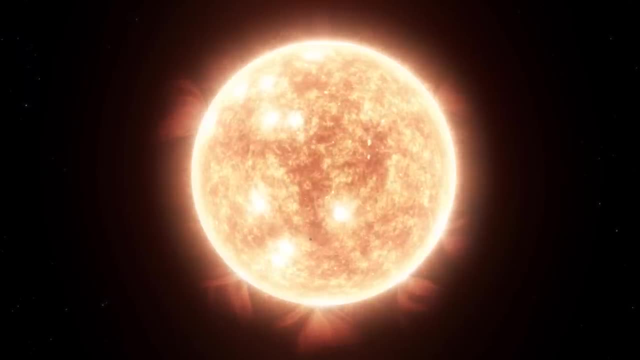 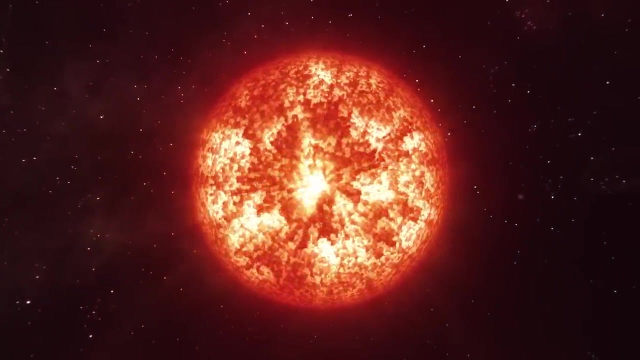 Mercury, which orbits the Sun at an average distance of about 58 million kilometers. Even if the star Gliese 581, is a rather low-luminosity star that is close enough to turn planet E into a hot desert world. Calculations showed that the planet would resemble Venus. 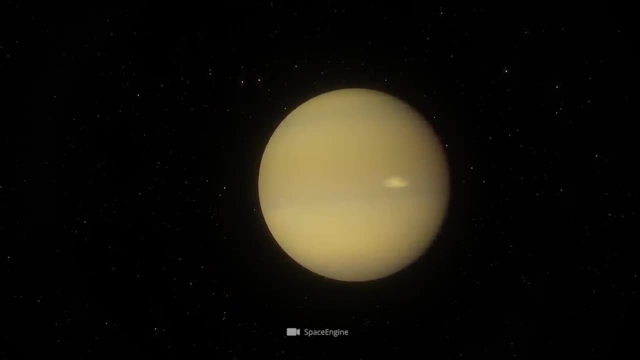 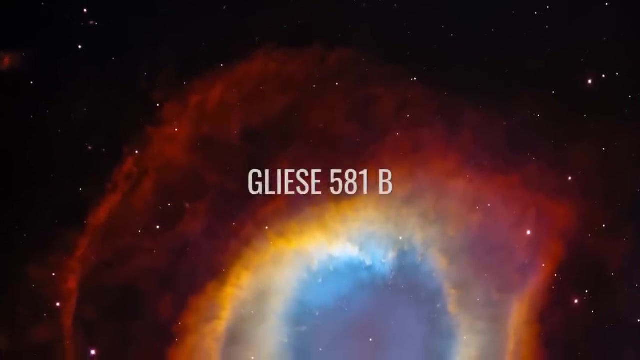 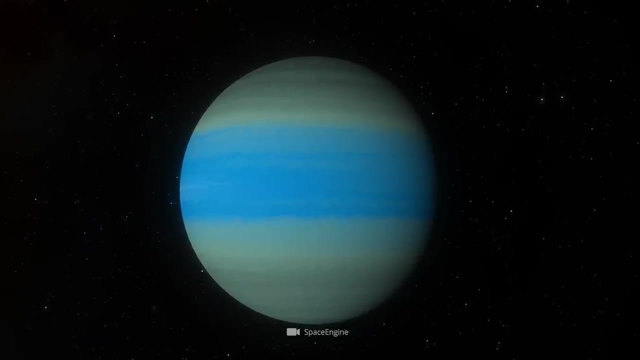 with surface temperatures above 500 degrees, There are probably only deserts on this planet, certainly no water and no life. Gliese 581b. The next planet in the Gliese system to cause excitement was Gliese 581b. This planet was initially classified as an Earth-like and warm world Surface. 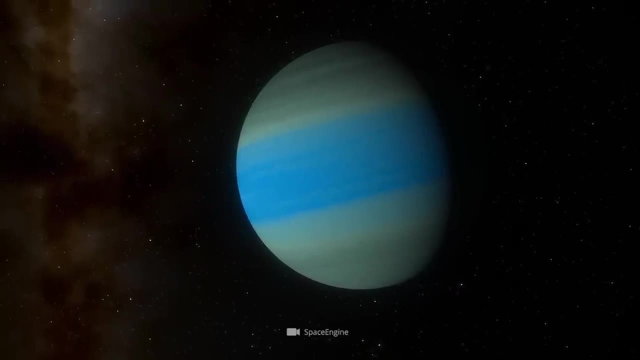 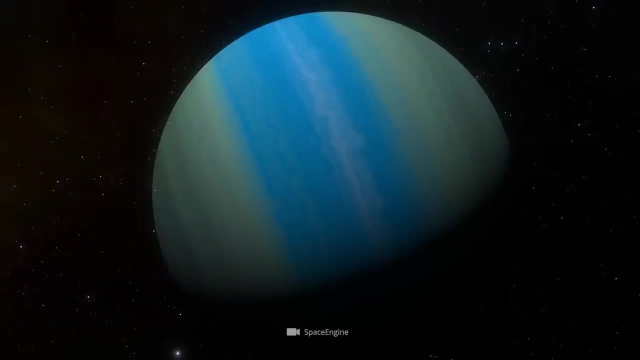 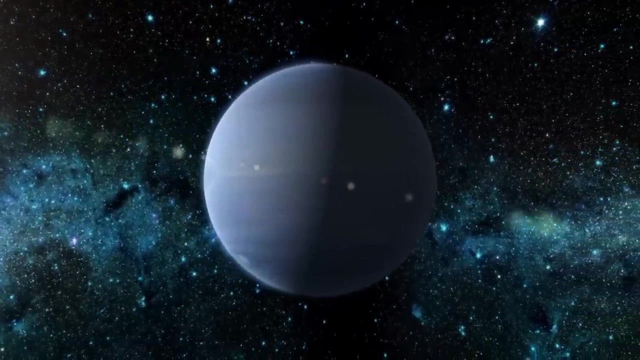 temperatures could range from 30.4 to 187 degrees Celsius. Later calculations came to a different conclusion. When it became clear that this planet has about 15.8 Earth masses, it became unlikely that it's a rocky world. Presumably Gliese 581b is. 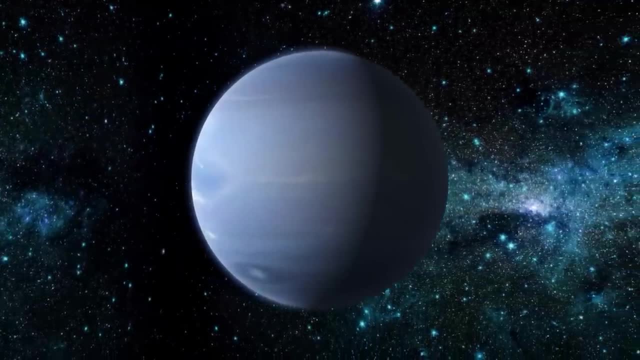 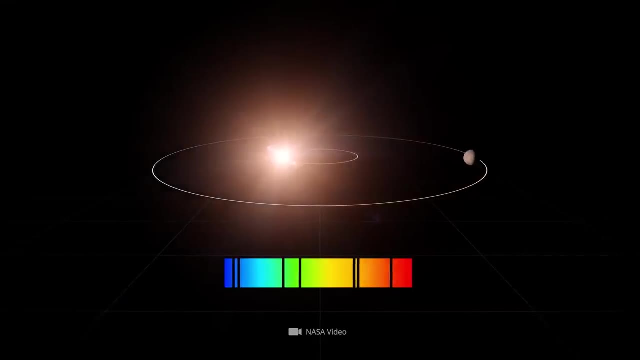 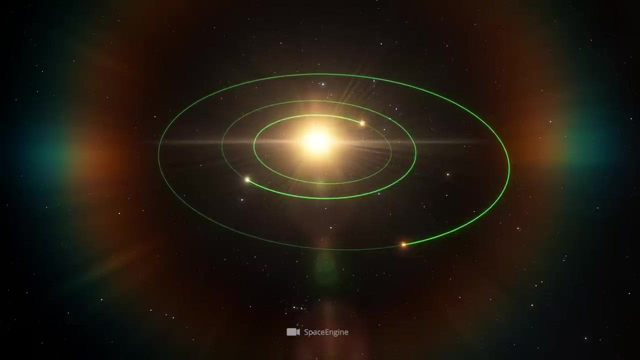 also much colder and could resemble the ice giant Neptune. Gliese 581 c. Gliese 581 c was discovered in 2007 using radial velocity methods and is a third safely detected exoplanet in the Gliese system. After the discovery of this planet, it was 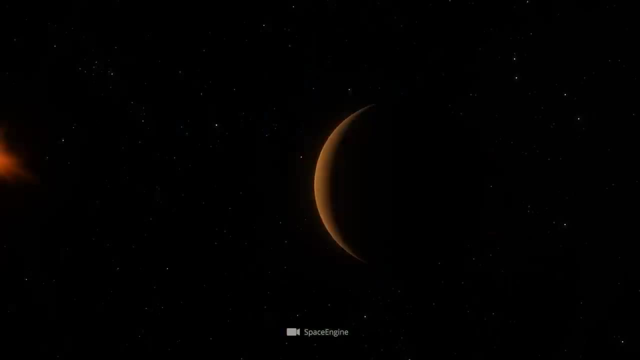 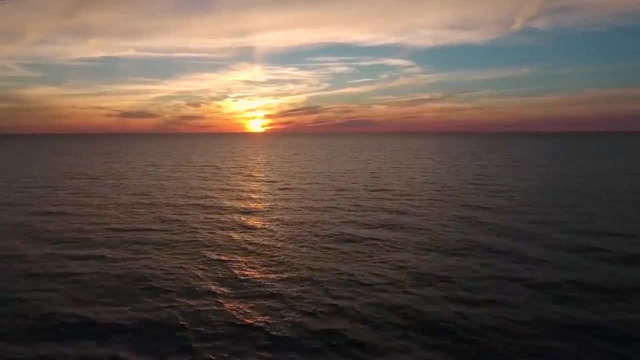 announced that it was a rocky planet in the habitable zone of its star, making Gliese 581c a hot candidate for the discovery of extraterrestrial life. Exoplanets in the habitable zone may have liquid water and likely have a climate conducive. 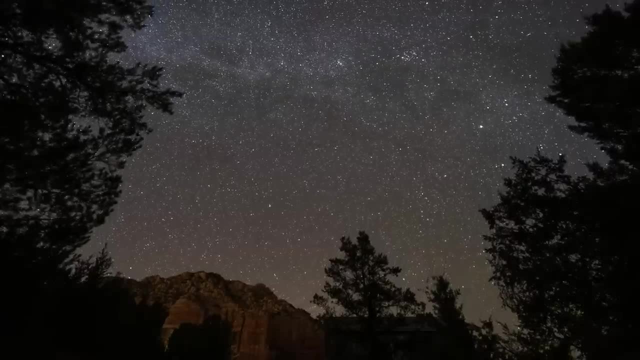 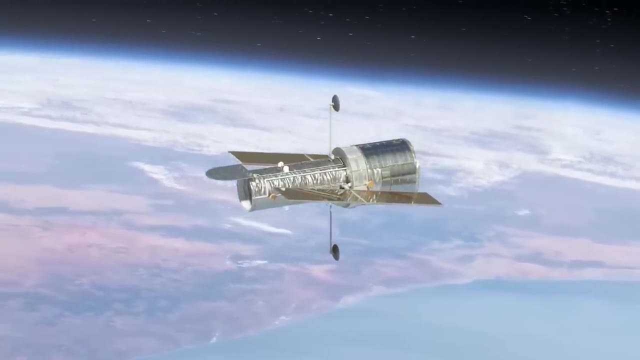 to the emergence of biological life. But we on Earth can't possibly know what planets are really like and unfortunately, no telescope in the world is currently capable of looking at their surfaces. The easiest way to spot possible intelligent life forms on a planet like Gliese 581c is 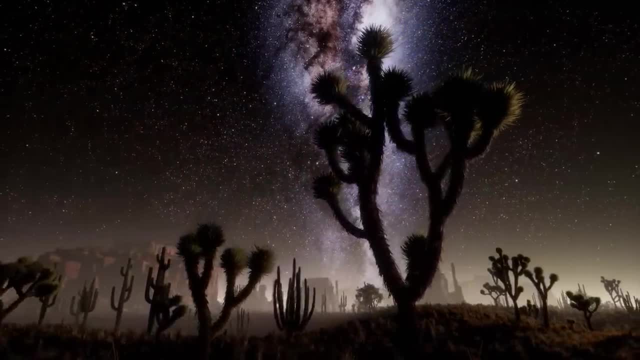 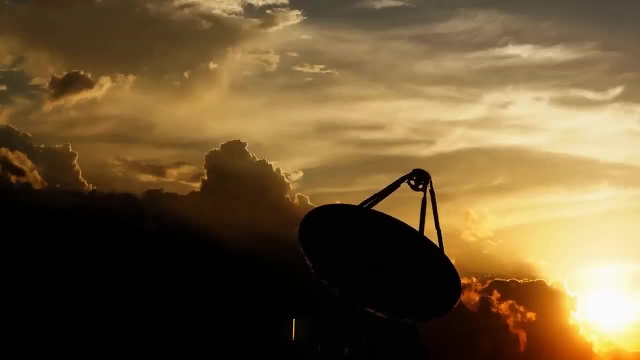 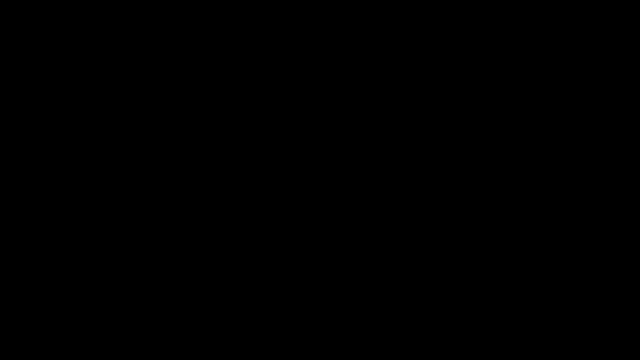 of course, to send a greeting message, which is exactly what they thought in Ukraine. a few weeks after the release of the sensational data, Ukrainian astronomers, using the giant RT-7 radio telescope, transmitted a radio message aimed directly at the exoplanet. 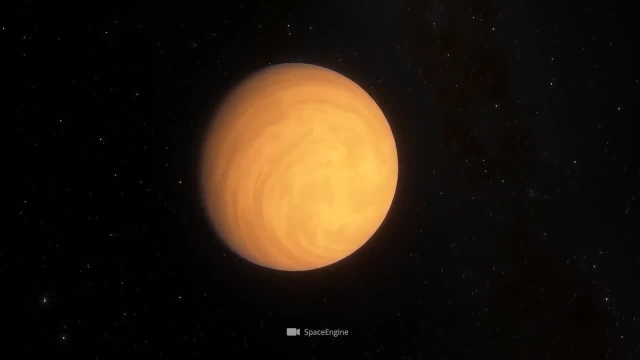 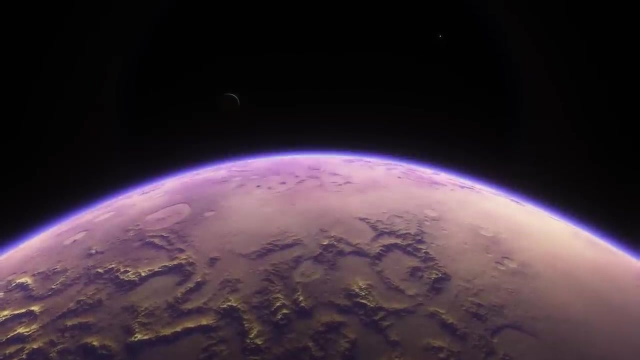 Only a short time later, however, an American group of astronomers announced that errors had been made In determining the facts surrounding Gliese 581c. the potentially habitable rocky planet which was supposed to be about five times larger than Earth, suddenly became a gas planet. 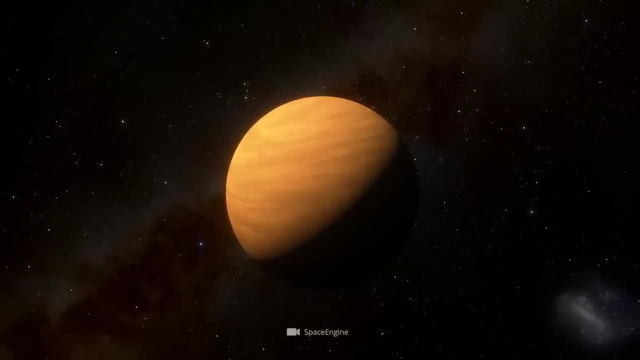 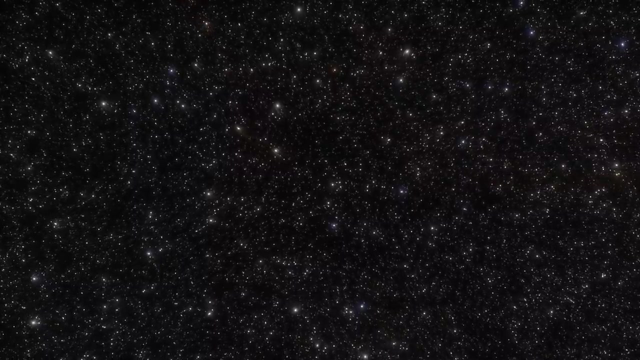 of 12.5 Earth masses, probably more like a small Jupiter, The prospects of finding life there faded away. The radio message of the Ukrainians is currently still on the way and will reach Gliese 581c in the year 2029.. 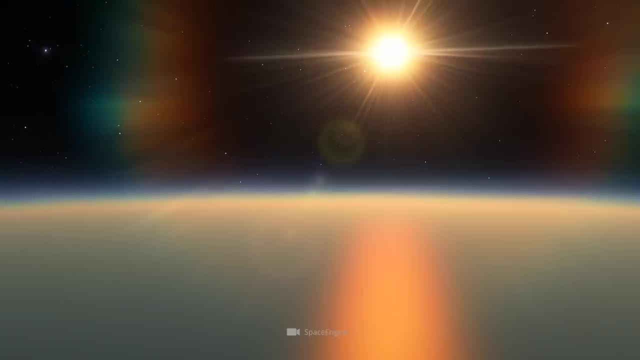 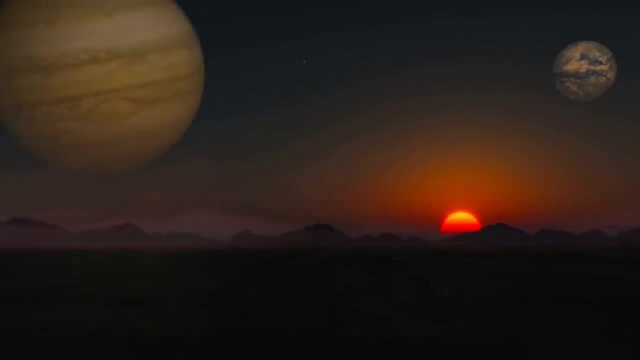 If someone did answer, it would be another 20 years or more before the reply reached us. After this failure, the frustration among scientists was great. But no life in the Gliese system. Astronomers were not going to be discouraged that easily. They pointed out that the planets in the Gliese system could have moons, and these too are potentially habitable celestial bodies. In our own star system, Saturn's moon, Titan, has long been thought to be a habitable world, And to this day it is not fully understood whether there may be methane-based bacteria. 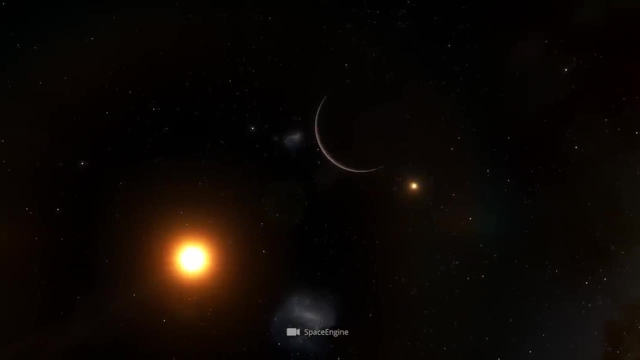 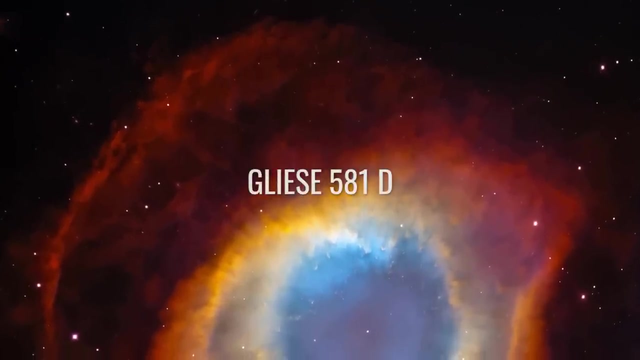 on the moon. In fact it is not a matter of fact, but of course it is a matter of fact. Other planets were discovered in the Gliese system and we do not want to withhold them from you. Gliese 581d. 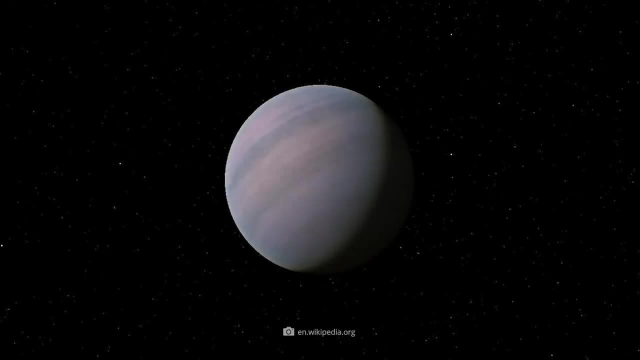 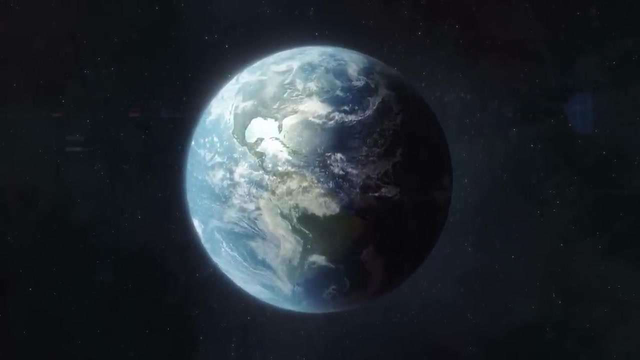 Only two years after Gliese 581c, the exoplanet D was discovered. When Swiss researchers came to the conclusion that this exoplanet could also be an Earth-like rocky world, the Gliese system was considered a super habitable solar system. 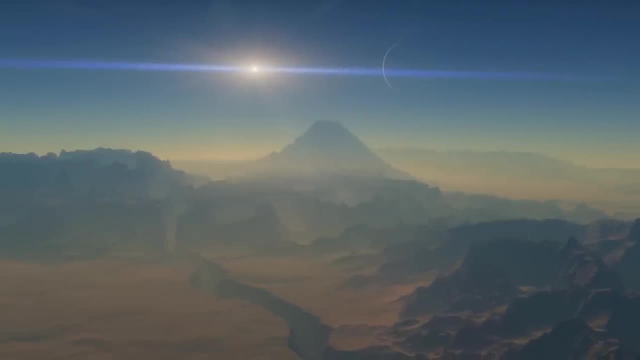 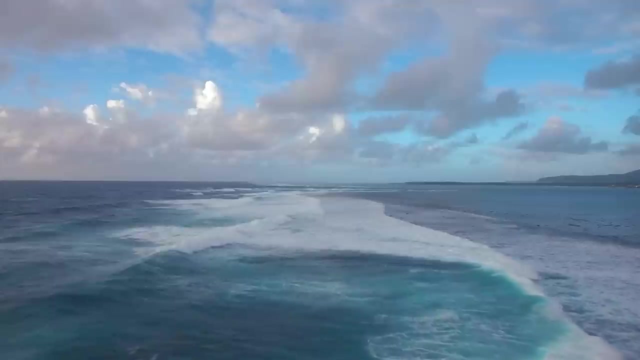 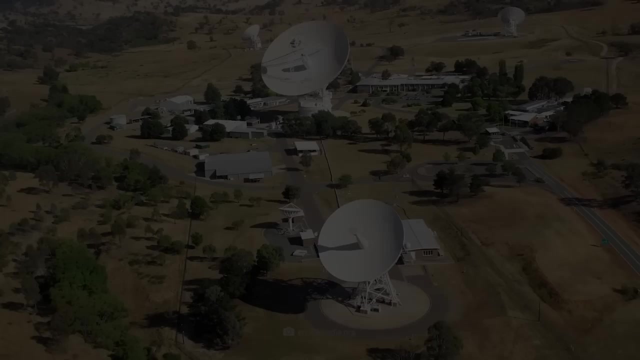 Two Earth-like planets appeared only too beautiful. Initially, everything was right. The planet moves within the habitable zone of its star, is about seven times larger than the Earth possibly, has oceans, rain and an atmosphere- All in all, perfect conditions similar to the Ukrainians. 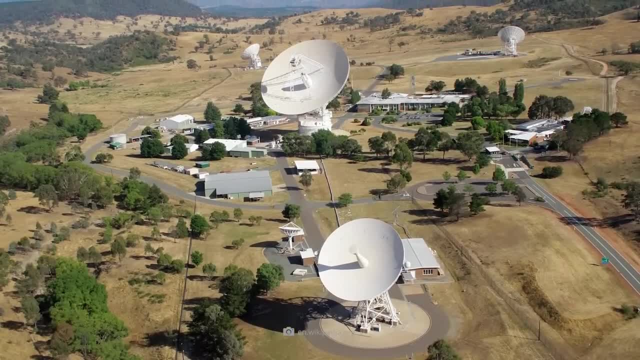 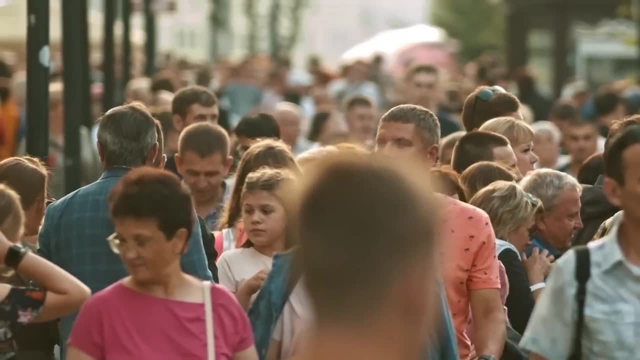 This time, scientists from the Kambara Deep Space Communication Complex sent a message directly to our supposed neighbors. In a large-scale campaign, people from all over the world were able to send 160-character texts to greet Gliese 581d and possible inhabitants. 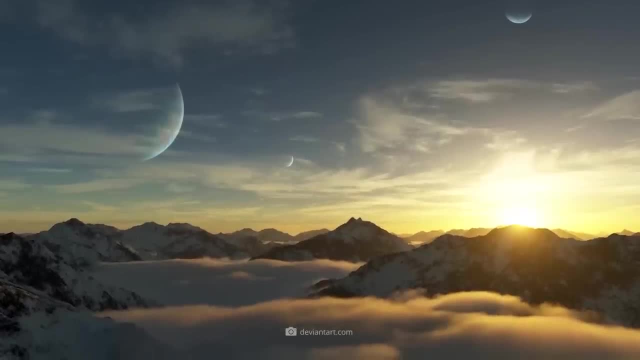 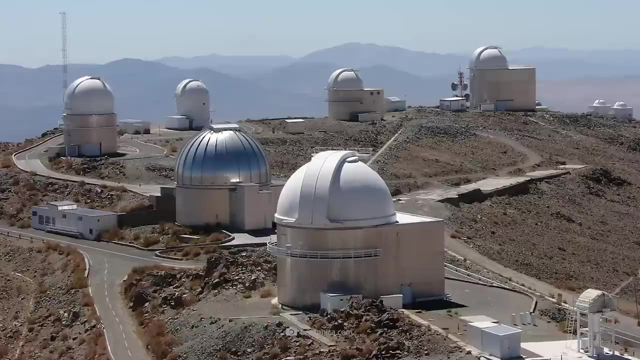 But also it was not easy. Also here, many thousands of people experienced a bitter disappointment. Checks of the data to this planet showed up that it possibly does not exist at all. Gliese 581d was originally discovered with the help of the HARPS instrument of the European 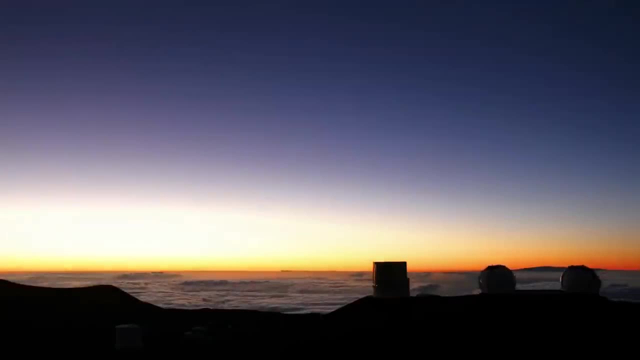 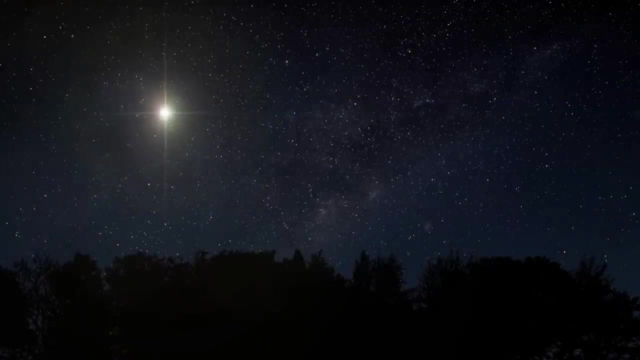 Southern Observatory In 2014,. researchers detected an error in the signal interpretation and the exoplanet did not fare well. Simply put, a small jolt from the star may have led astronomers on Earth to think they could find evidence of its existence. 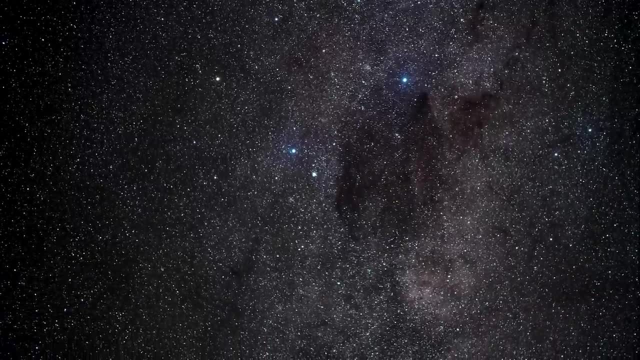 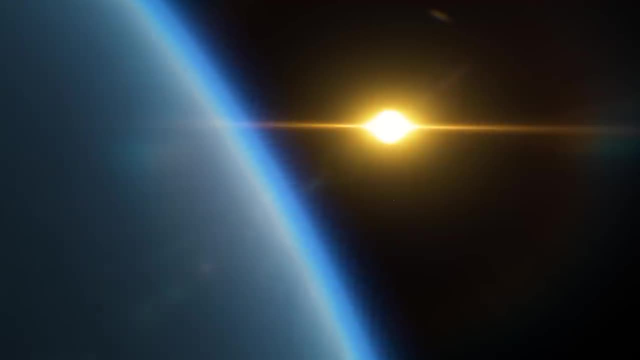 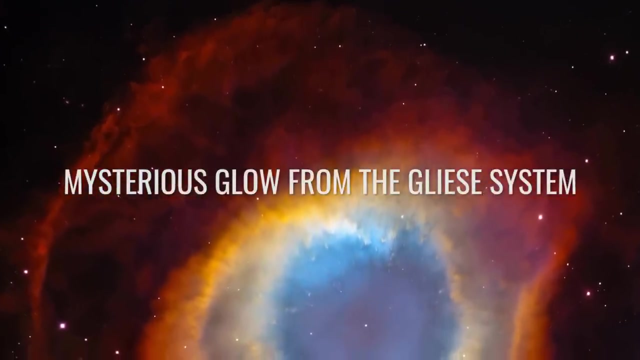 However, there is no evidence of a planet in the motion irregularities. The same was true for Gliese 581f and G. Only the existence of the first three presented planets was confirmed for sure. All others are not sure until today. Mysterious Glow from the Gliese System. After the announcement of the discovery of 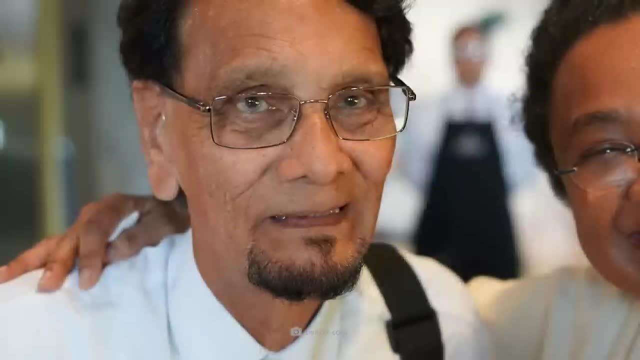 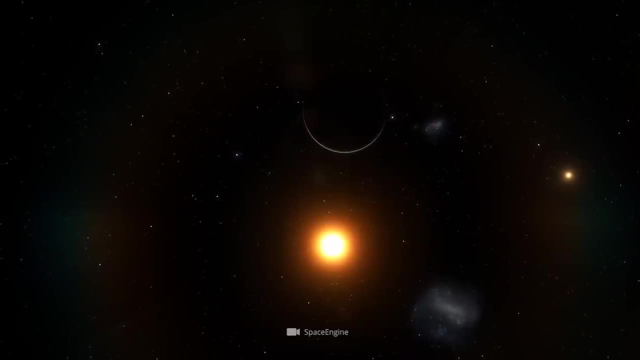 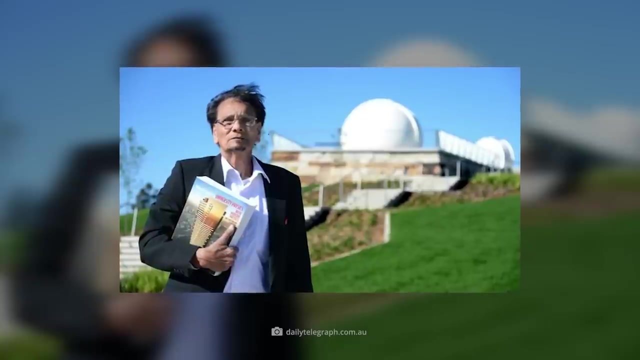 Gliese 581g on September 29, 2010,. an Australian astronomer named Radbir Bathal claimed to have detected a suspicious pulse at the exact position of Gliese 581g two years earlier. Bathal is a member of the Australian branch of SETI, a non-profit scientific organization. 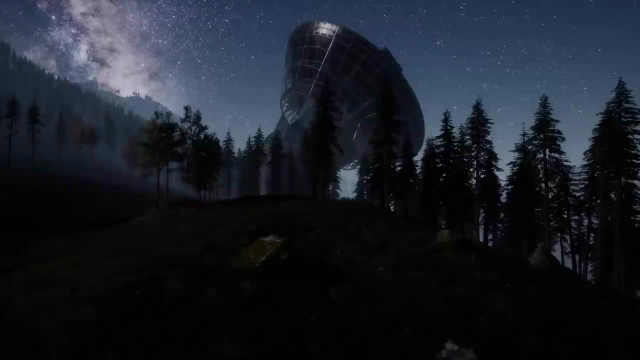 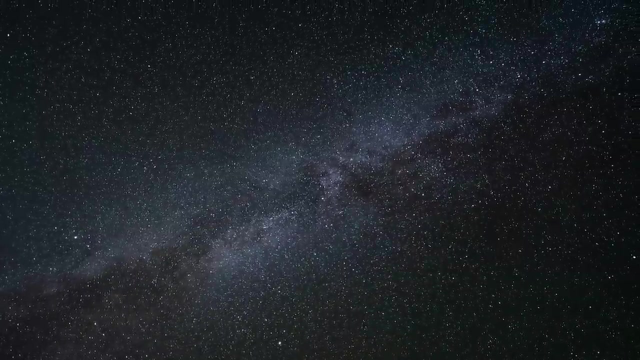 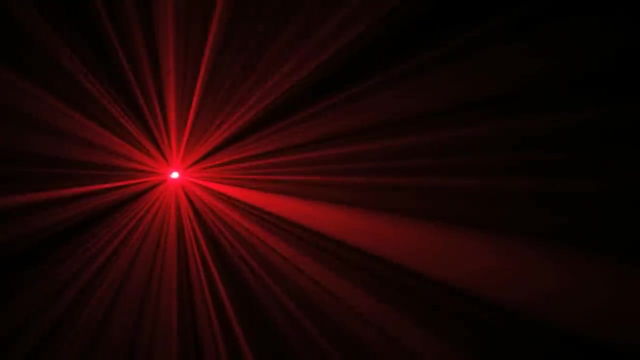 dedicated to finding technosignatures in space. These include any signals that might emanate from technological devices, or in other words, radio transmissions, radio waves of non-natural origin, traces of vehicles moving through space, and so on. Bathal claimed that the signal pointed to an artificial light source similar to the. 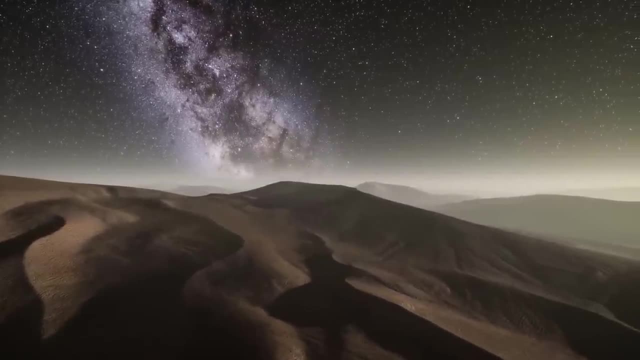 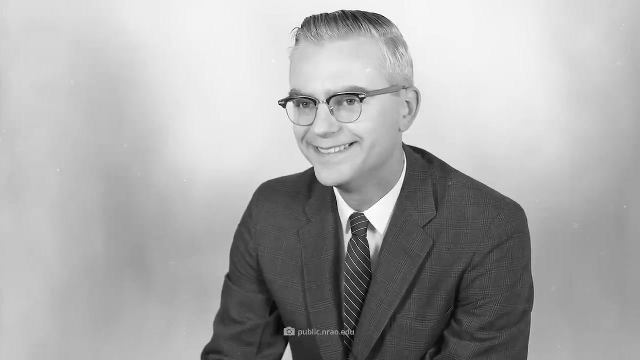 tip of a laser light. After this sensational news, researchers naturally wanted to verify the information. None other than Frank Drake, the SETI pioneer, took up the case, But Bathal could not provide any data at first, and the evidence he sent to Drake after some. 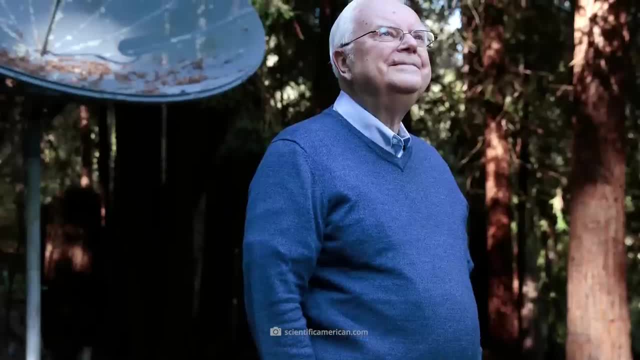 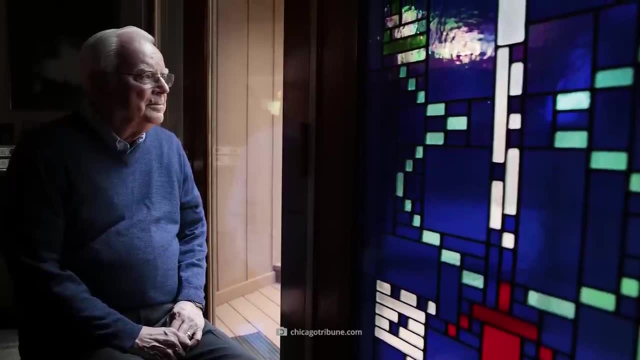 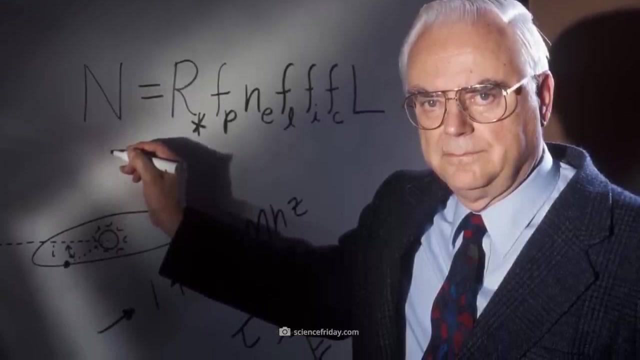 inquiries unfortunately did not convince the astronomer. Frank Drake commented to Spacecom, saying: I'm very suspicious. Drake sent the first signals to search for extraterrestrial intelligence into space 50 years ago. He also created the Drake Equation, which indicates how many intelligent extraterrestrial 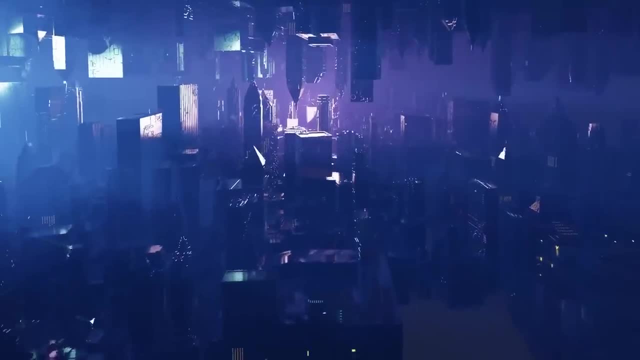 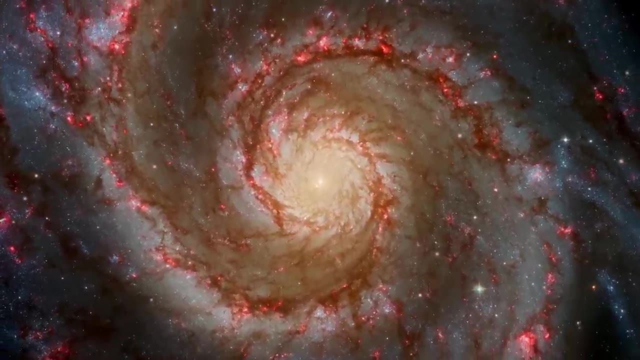 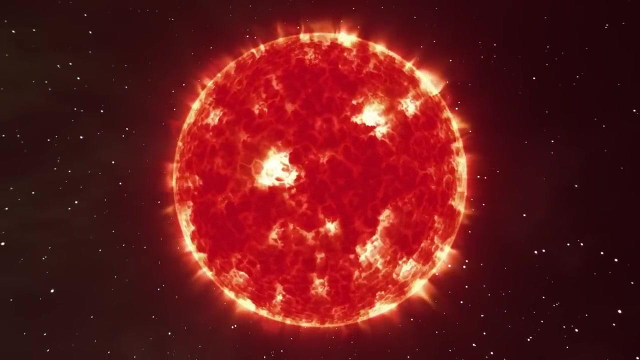 civilizations there must be in the cosmos based purely on statistics. Using the former, it was determined that there could be more than 300 million worlds with Earth-like conditions in the Milky Way alone. About half of the Sun-like stars must have rocky planets in habitable zones. 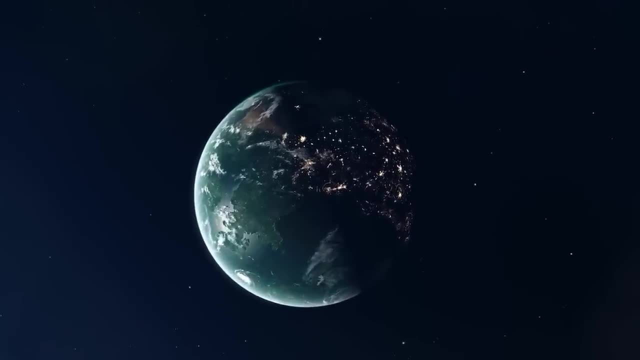 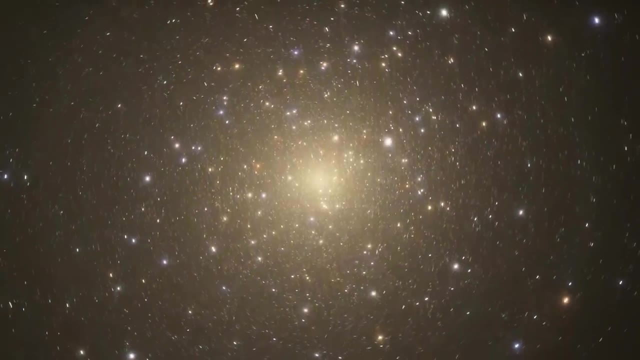 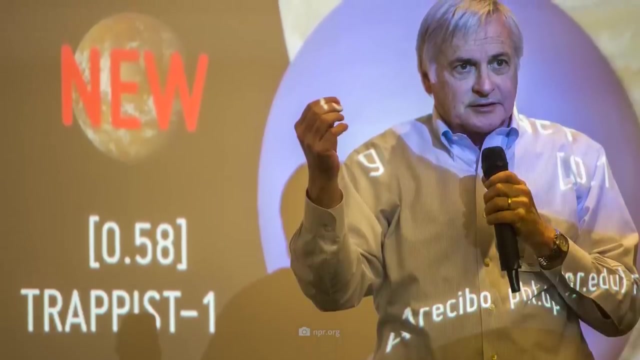 Then there is the question of how many of the potentially habitable planets are actually inhabited, and what kind of life forms are there and at what stage of development. Astronomers searching using the Drake Equation and similar concepts came up with 36,, while physicist Seth Shostak determined in 2018 that there could be 10,000 extraterrestrial. 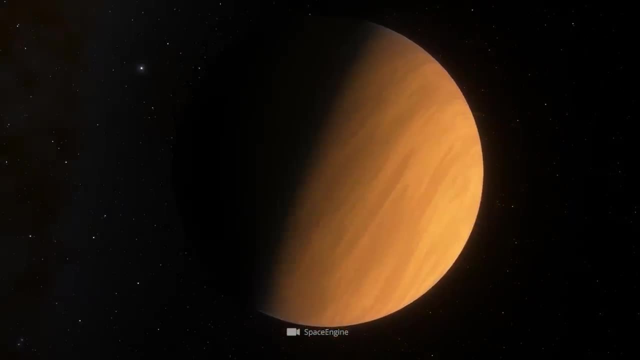 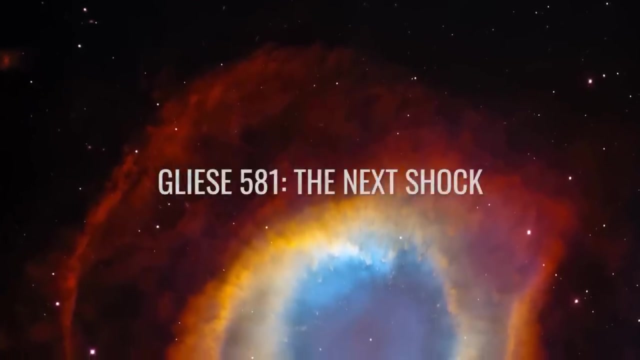 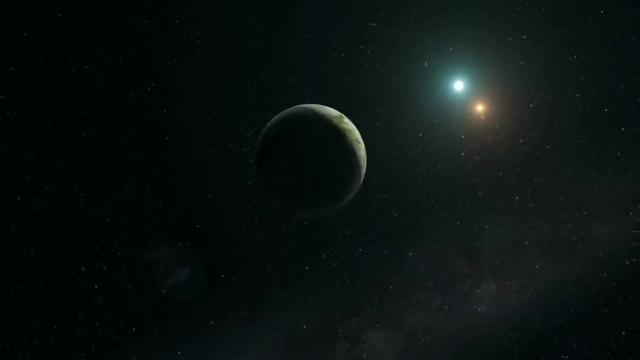 civilizations in the Milky Way. That one of them is native to the Gliese system, however, is now almost impossible, And we'll show you why. Gliese 581 – The Next Shock. Despite the failures in the Gliese system, astronomers were not deterred from continuing to study the star and its planets in detail. 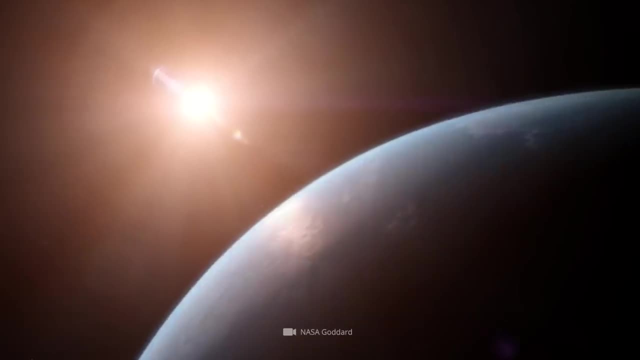 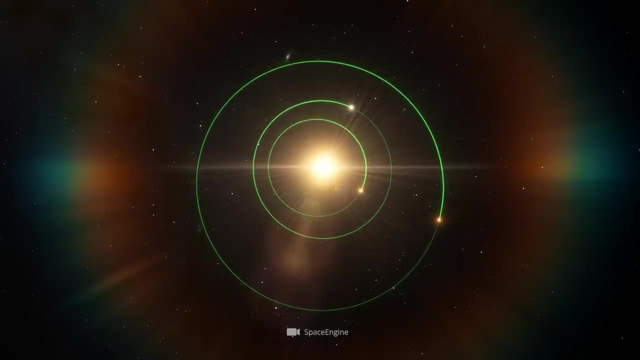 With improved measuring techniques and renewed calculations, at least the data of the first three exoplanets should be confirmed. While these studies were going on, something happened on the star Gliese 581 that again deeply shook the world of science. The red dwarf unexpectedly blew gigantic flames. 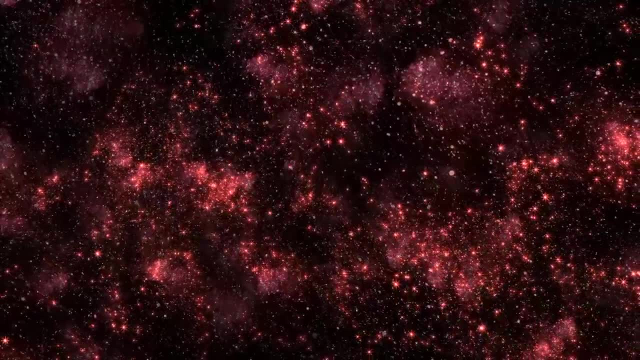 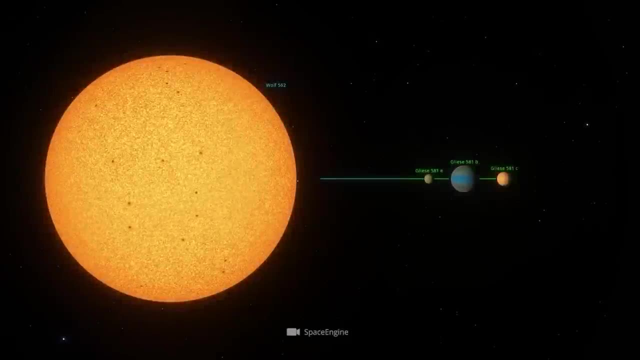 The red dwarf unexpectedly blew gigantic flames. The red Baron instantly flashed flares into its environment With the particle storms. such large quantities of cosmic radiation might have reached the direct environment of the star that the hopes that any of the 3 confirmed planets might